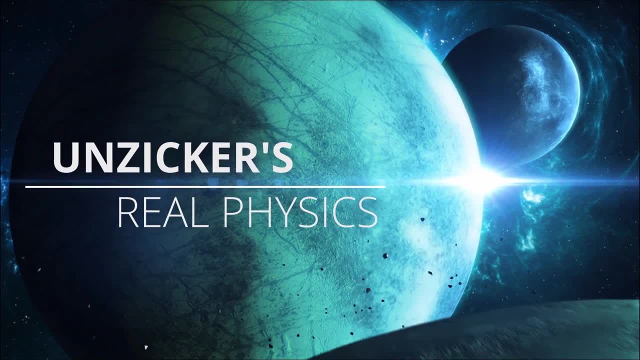 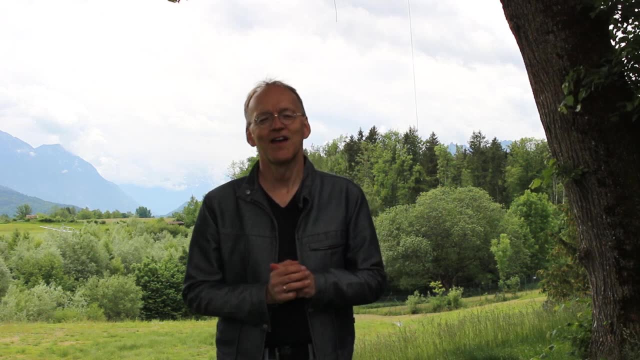 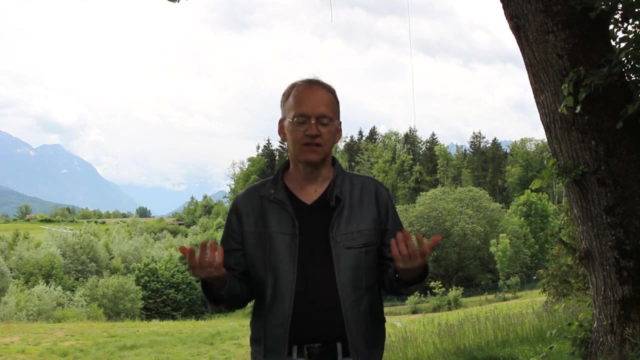 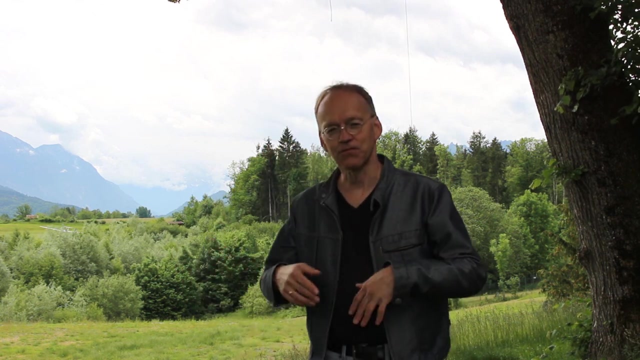 Welcome to Real Physics. This is a series of short clips about misleading concepts in physics, and today I'm talking about the weak interaction. What is weak interaction? Well, it's not even interaction. It's not even a force, because you have the force of gravity with a well-known 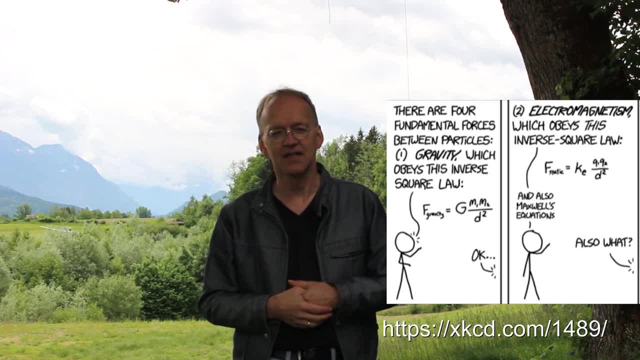 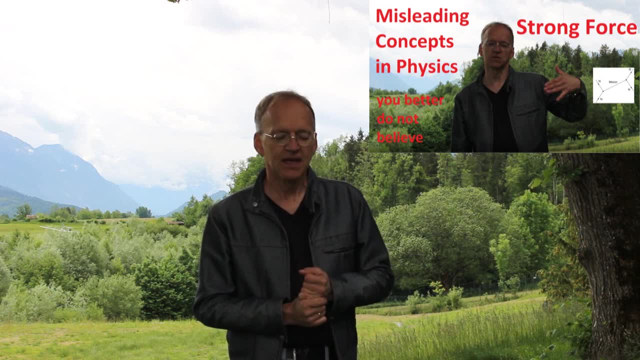 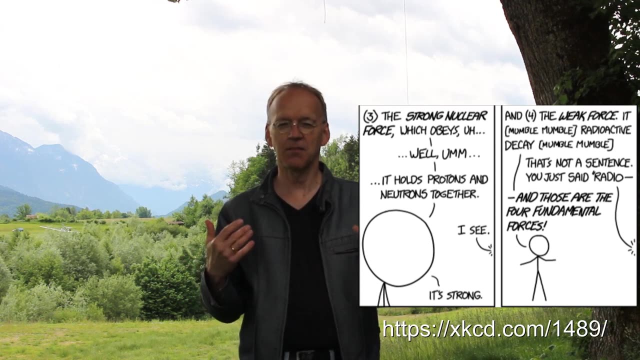 1 over r, squared dependence, and the same with electrodynamics. and then you have the so-called strong interaction, which is questionable, as I explained in another video, But there was at least the idea for force. but at the weak interaction there isn't even a force. It's somehow related. 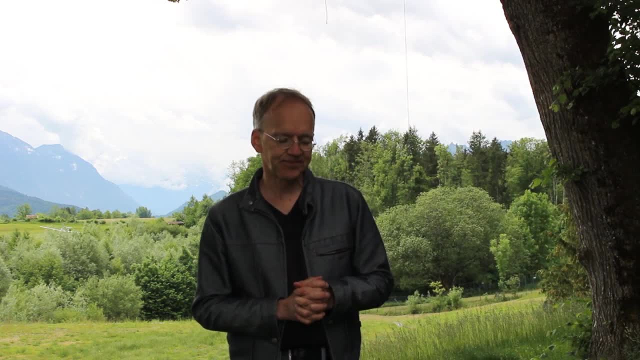 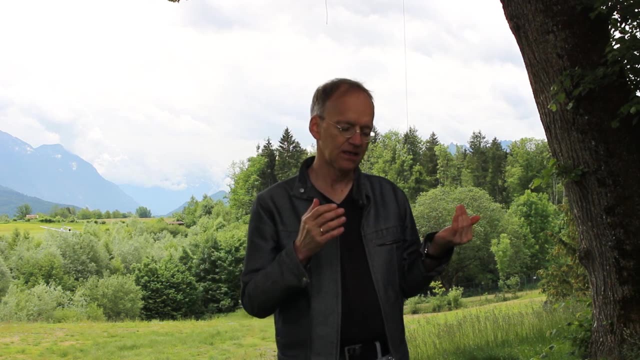 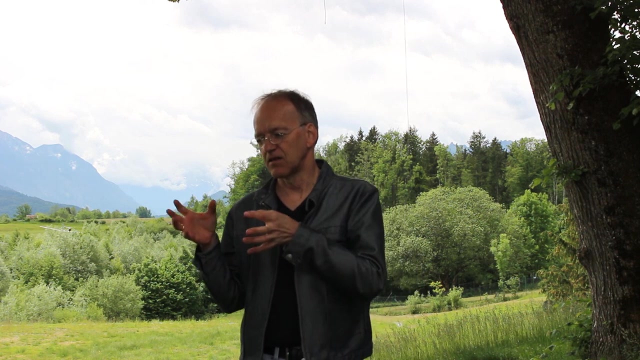 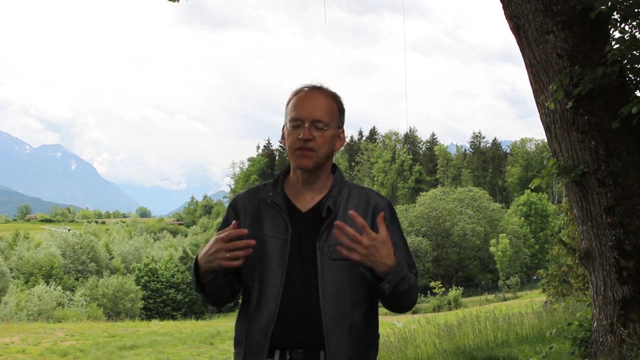 to beta decay. and well, what's the difference between strong and weak The interaction of the nucleus? they take place on a very short time scale and the beta decay takes place at a relatively long time scale. So there is something very different in these two processes. and then you 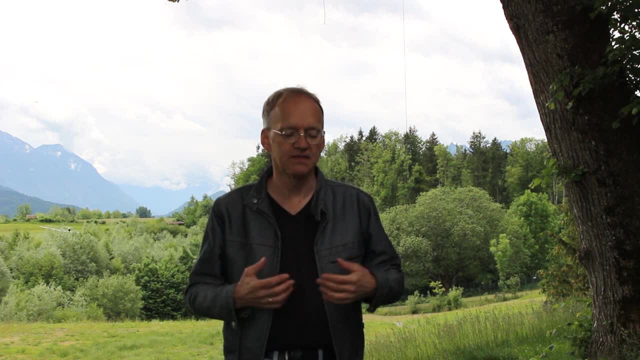 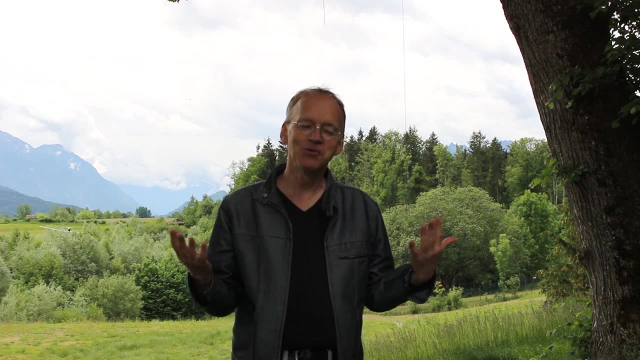 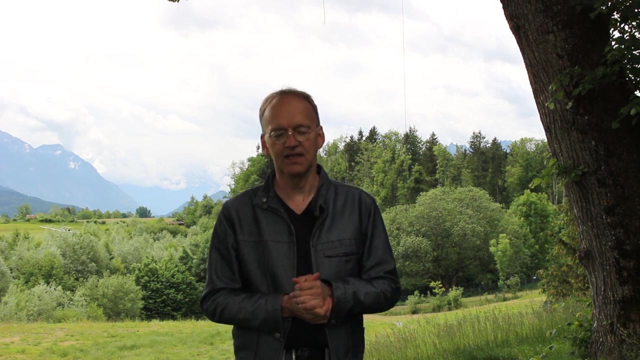 have. they have coined two different terms for it. That's the reason. Okay, but whenever you hear something new, it's very often that you hear something new. It's very often that you hear something that there is something behind you don't understand, and the thing we do not understand is beta decay. 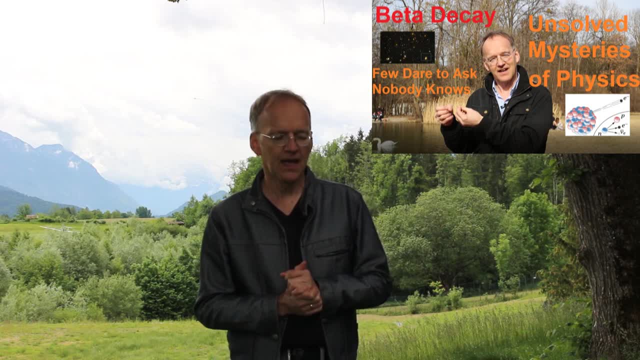 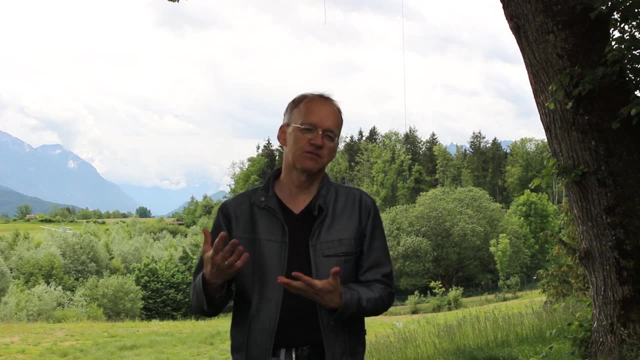 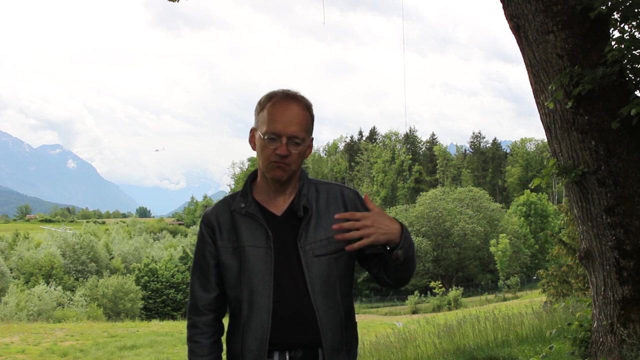 I made another video about this riddle, and there are lots of unsolved problems which today's physicists are just glossing over by inventing new names, and but one of the very, very principal missteps, I think, was the the introduction of this weak interaction. 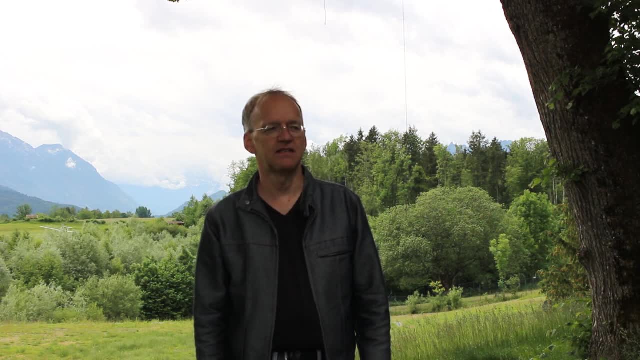 Does the weak interaction have a negative effect on the interaction? Well, it doesn't. Does the weak interaction have a negative effect on the interaction? Well, it doesn't really make sense. and if you want to advance physics, you, you should not postulate a strong. 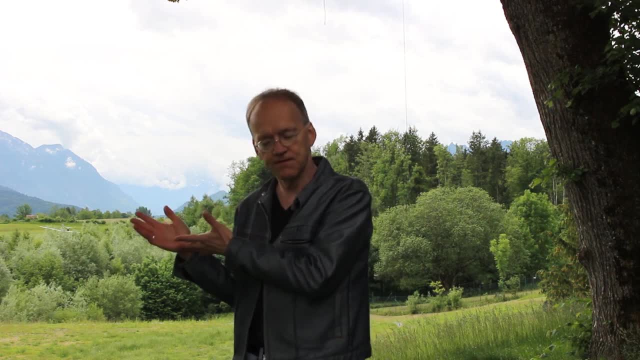 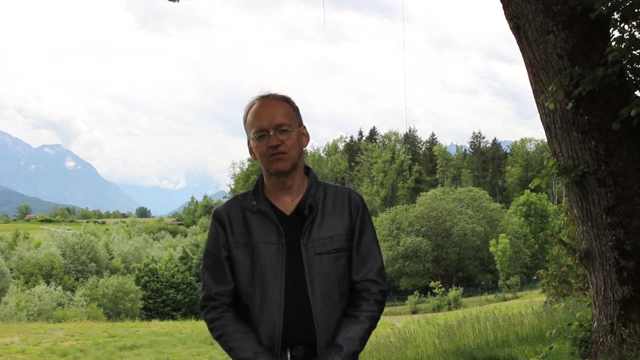 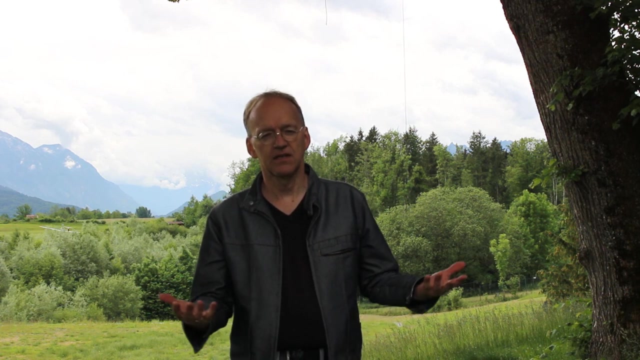 and weak, or a third and fourth and maybe fifth force, but to think about how to unify the two existing forces, gravity and electrodynamics, and, as I said in the other video, the great physicists of the beginning of the 20th century. they wouldn't even consider the idea they were.